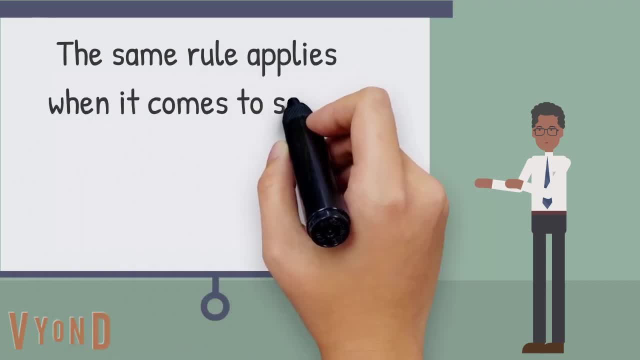 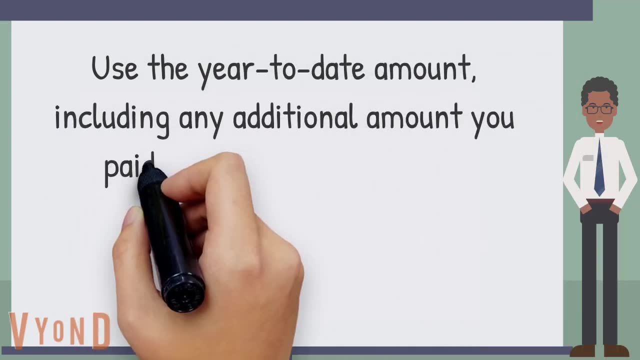 wages not included in the pay stub you are using. The same rule applies when it comes to Social Security and federal withholdings. Use the year-to-date amount, including any additional amount you've paid throughout the year, to determine the appropriate number to enter into the online calculator. 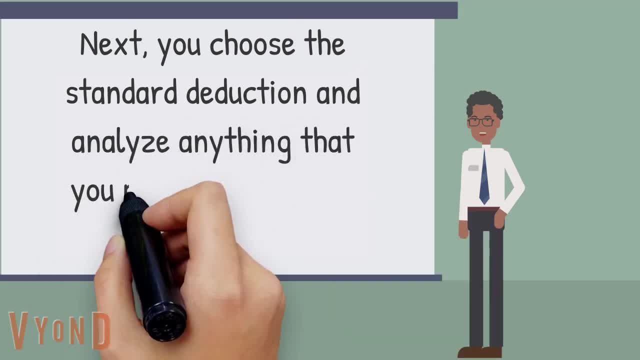 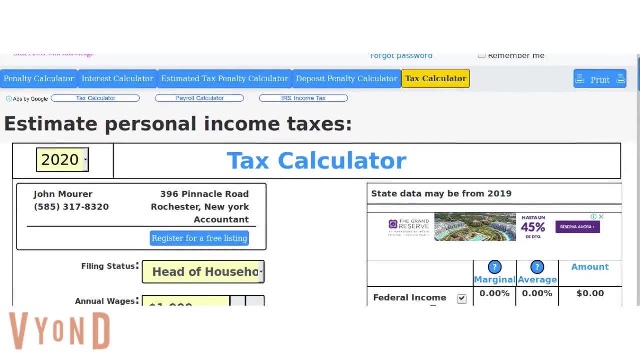 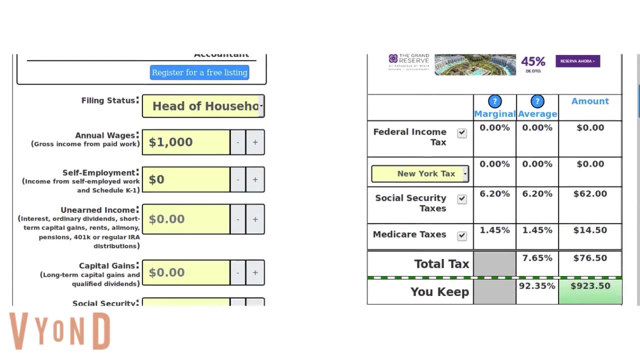 Next, you choose the standard deduction and analyze anything that you plan to itemize as part of your deductions. Online Tax Estimation with the IRS Calculator. Here is the online calculator for you tax estimation. You need to fill the information and look at how it automatically calculates the relative taxes. 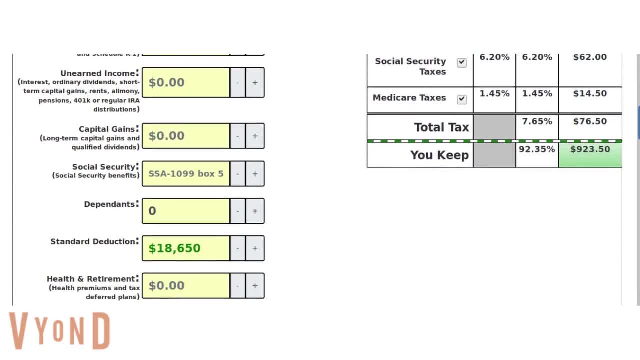 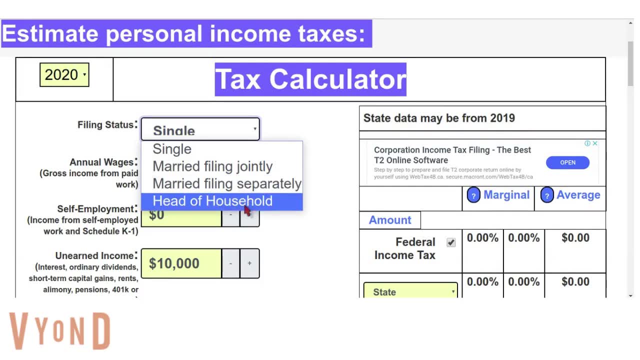 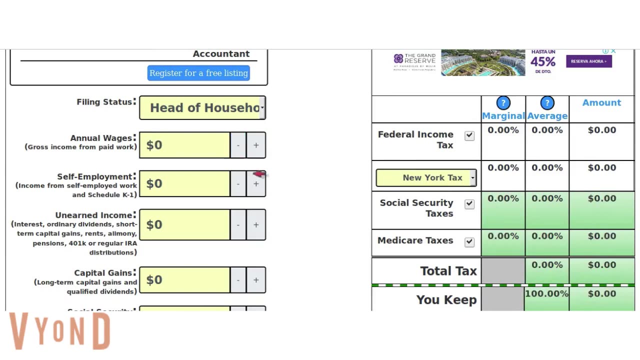 Input on the left side is about your information. In the right side you can see the tax calculation Filing status. You can input your annual salary as an employee or independent contractor. You can see your yearly income on the pay stubs, year-to-date section. 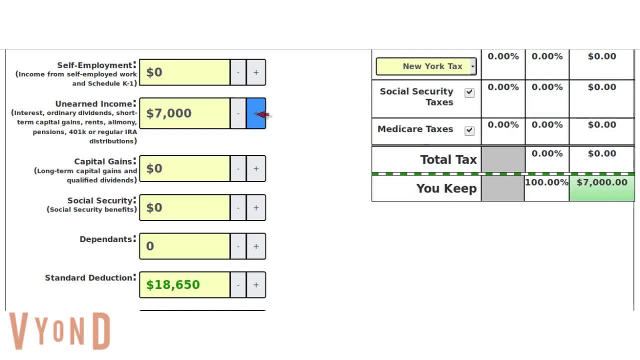 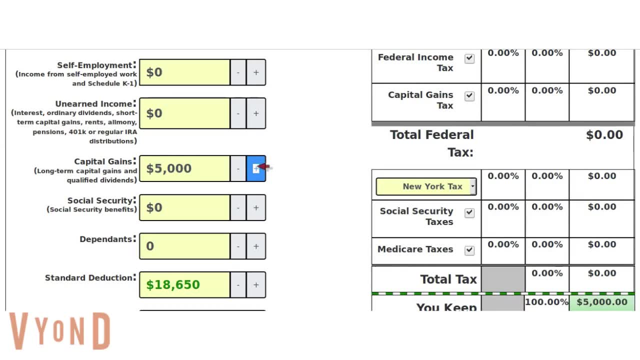 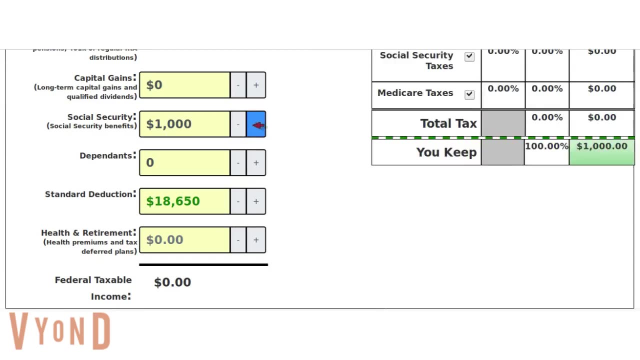 Unearned income and capital gain is the money you make from interest: ordinary dividends, short-term capital gains, rents, alimony pensions, 401k or regular IRA distribution, Long-term capital gains and qualified dividends dividends. Some of you have to pay federal income taxes on your social security benefits. 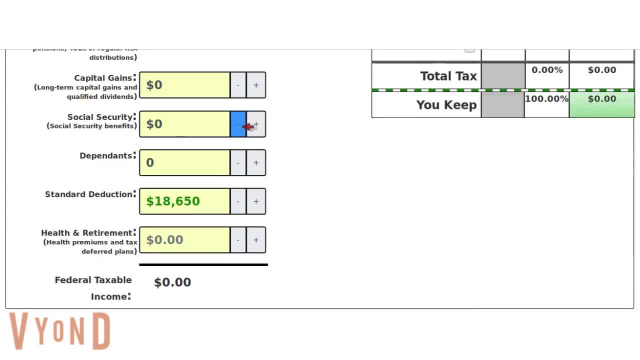 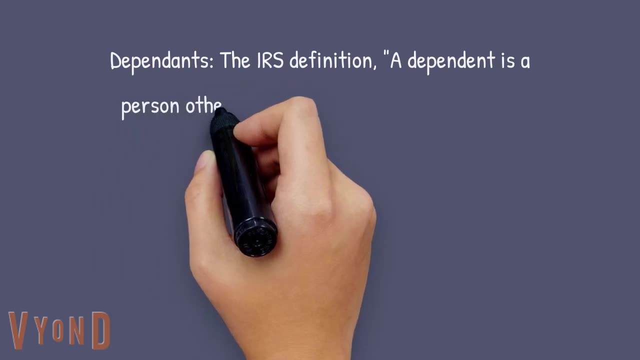 Between $25,000 and $34,000, you may have to pay income tax on up to 50% of your benefits. More than $34,000,, up to 85% of your benefits may be taxable. A dependent is a person other than the taxpayer or spouse who entitles the taxpayer to claim a. 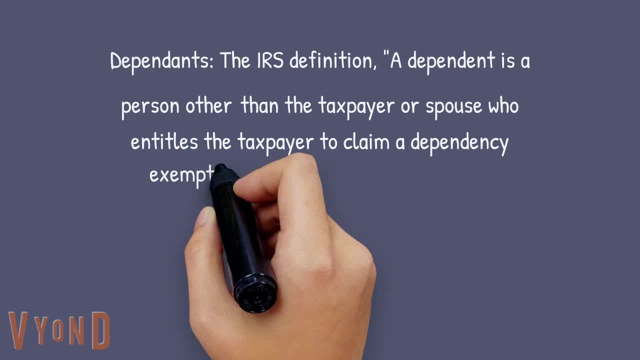 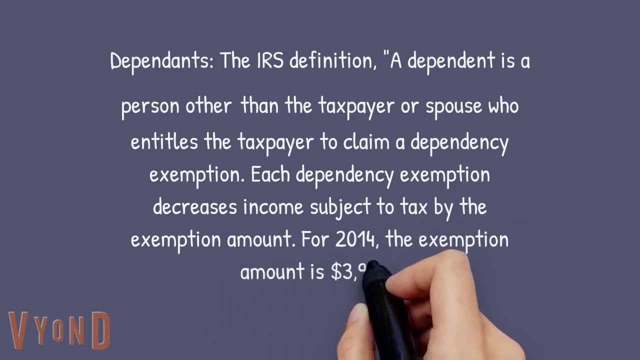 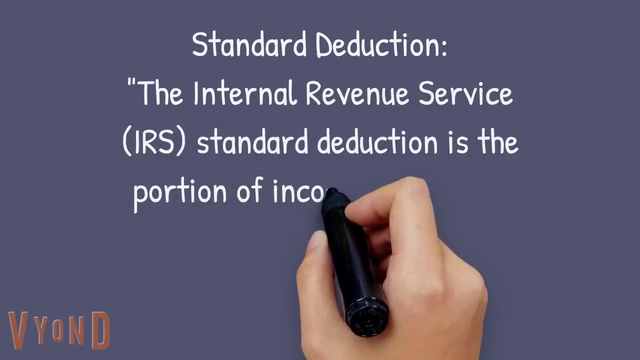 dependency exemption. Each dependency exemption decreases income subject to tax by the exemption amount. For 2014,, the exemption amount is $3,950.. Standard deduction: The Internal Revenue Service IRS. standard deduction is the portion of income that is not subject to tax that can be used to reduce your tax bill. 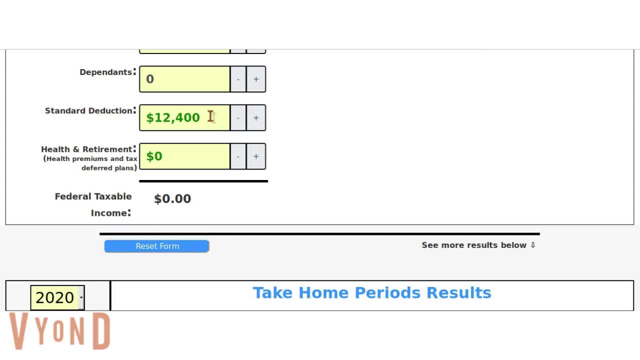 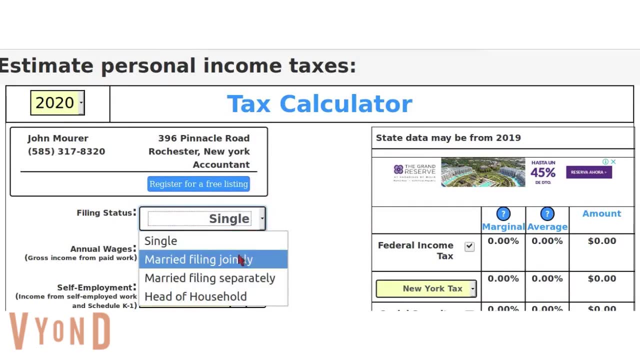 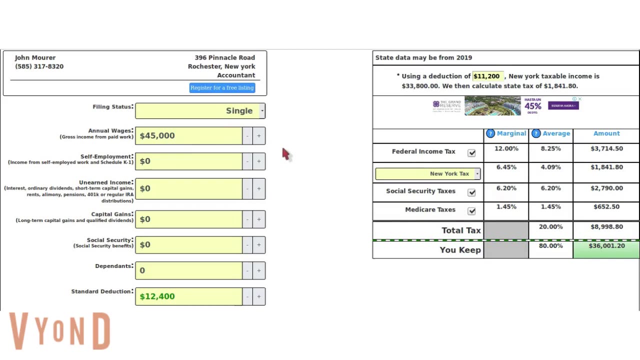 Changing the filing status will change your standard deduction. You can see how it has changed from a single- $12,400.. To a married filing jointly $24,800.. We can see how the single filing status that has an annual wage of $45,000 will end paying taxes.